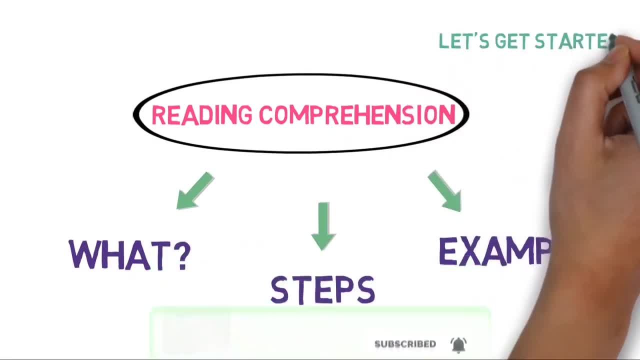 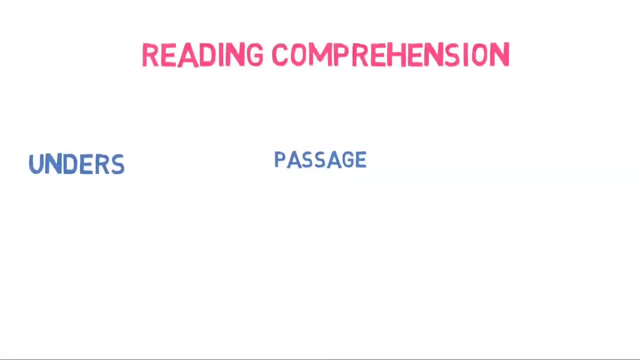 So, without further ado, let's get started. What is reading comprehension? Reading comprehension is the ability to understand the content of the given passage and to draw a conclusion from it. Here the author will give his point of view from different angles for a particular topic. 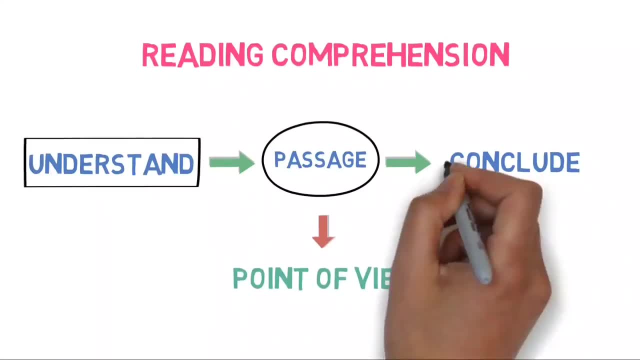 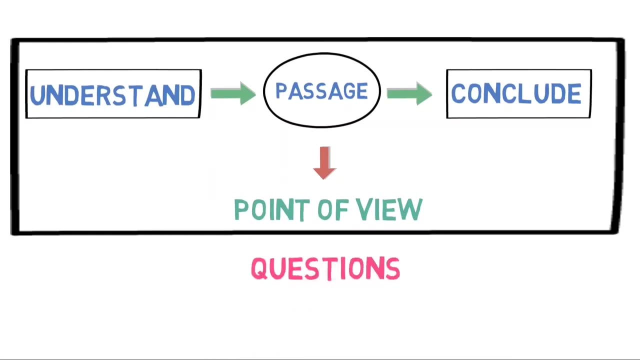 and you have to understand and to draw out a conclusion from it. To test what you have comprehended or understood from a passage, a set of questions will be given to you and you have to solve it. You must have strong command in vocabulary and grammar to understand reading comprehension. 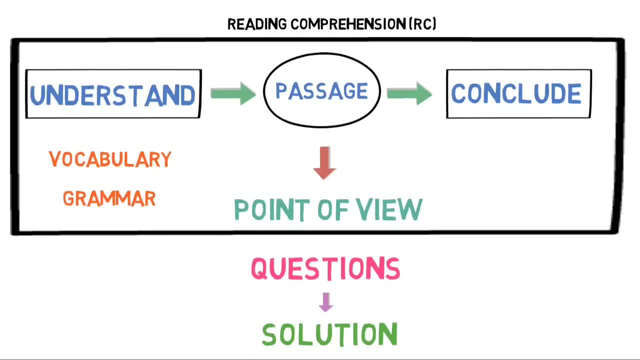 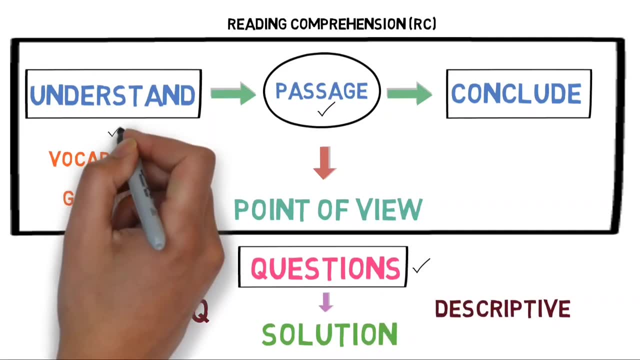 or in short, RC, and to solve this type of questions. There are two kinds of questions asked in exams: MCQ or multiple choice and descriptive. To sum up, you will be given a passage and questions based on that passage. You have to understand the passage, conclude it and solve the questions. 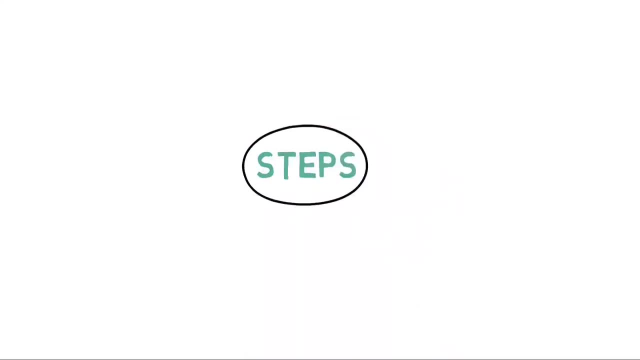 Let's learn the steps to solve the questions related to reading comprehension. There are three steps involved in solving this kind of question. 1. Scheme: Here you need to read the passage fairly quickly to get a general idea of what the author is saying. 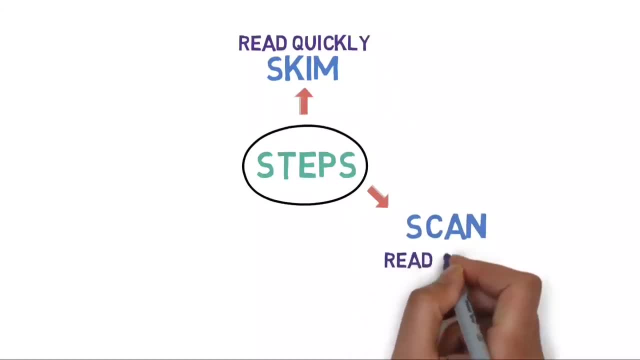 2. Scan: Read the passage again, this time in a slow manner, to know the details. Underline the key words and sentences. Also, you may create A quick mind map of the passage. 3. Solve: Take one question at a time. study the question thoroughly. turn to the relevant portion of. 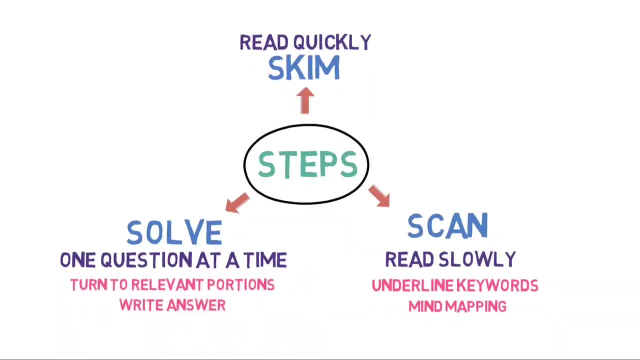 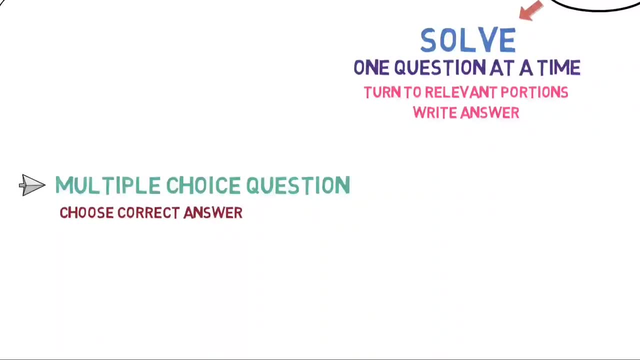 the passage. read them again and write the answer accordingly. For MCQ-based questions, choose the correct answers from the given answer. In case you are not sure about the answer, you may use a technique called intelligent guessing Here. If you made the wrong ones, re-read the part of the passage again and try to choose the 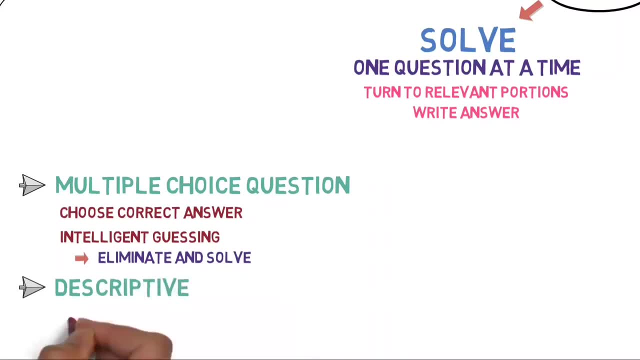 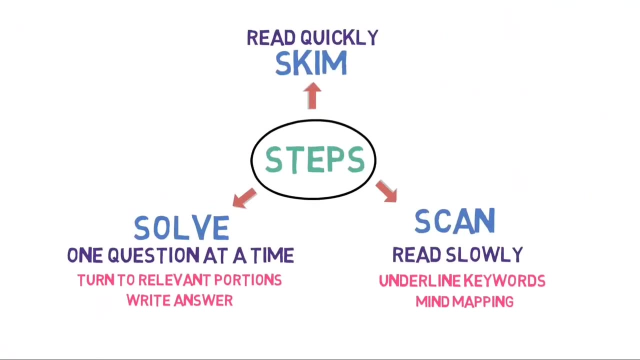 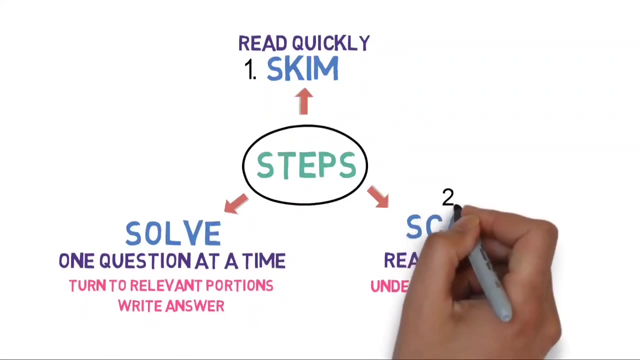 correct one For descriptive-based questions. write the answers in your own words, neatly and precisely. Once again, I will explain you the steps. 1. Scheme: Read the passage fairly quickly to get a general idea. 2. Scan. 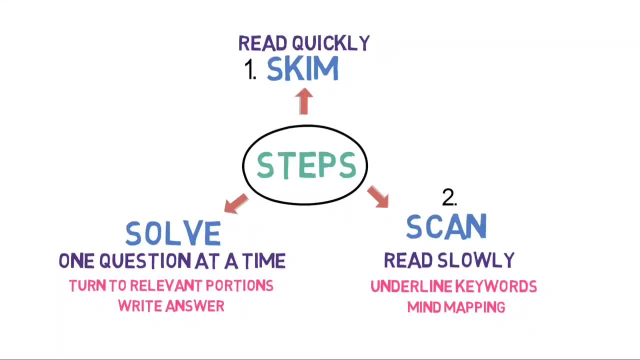 Read again, this time in a little slow manner, to know the details. 3. Solve: Take one question at a time. study the question thoroughly, turn to the relevant portion of the passage, read them again and write the answer. Now that you have understood the steps, let's understand the type of questions that might. 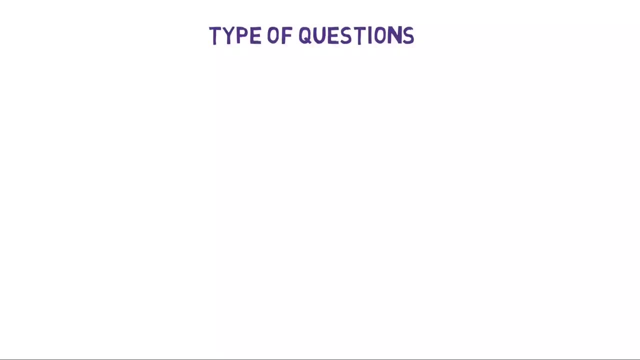 come in the exercise related to the reading comprehension: 1. Questions related to the central idea of the passage. 2. Questions related to the conclusion of a particular paragraph. 3. Questions related to the conclusion of a particular paragraph 4. 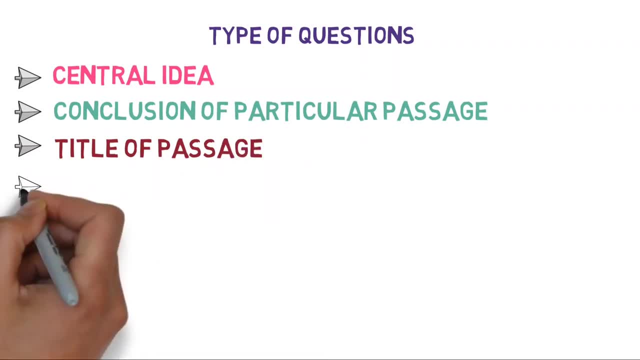 Questions related to providing the suitable title of the passage. 5. Questions related to vocabulary, like synonyms meaning similar words, antonyms meaning opposite words. 6. Questions on context of the passage. 7. Questions based on opinions and facts. 8. 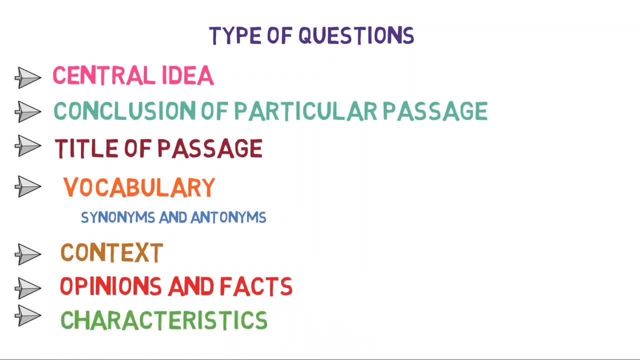 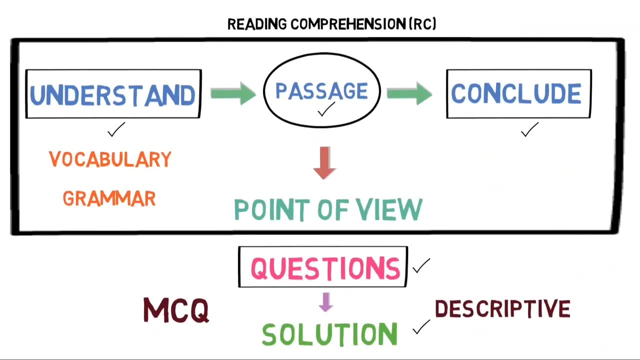 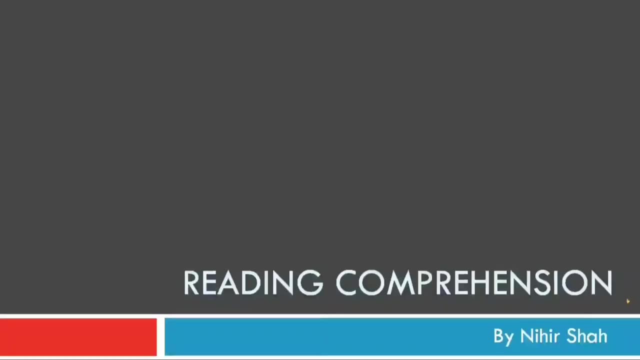 Characteristics of the writer. So these are some of the types of questions that might come in any reading comprehension. Now that you have understood what is reading comprehension, Now that you have understood what is reading comprehension, The steps to solve it and the types of questions that might come, let's look into an example. 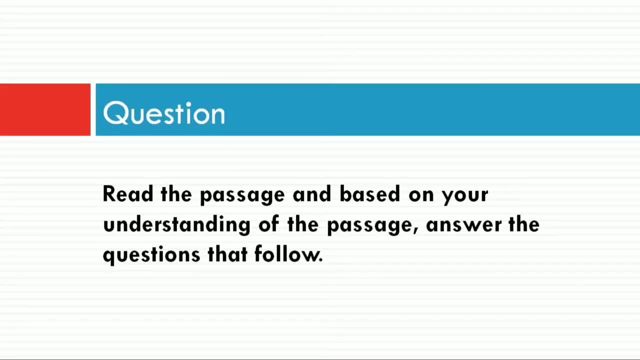 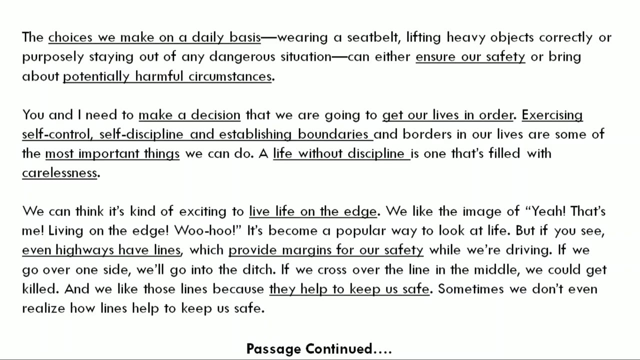 of it The question is. read the passage and, based on your understanding of the passage, answer the questions that follow. While I will go through the slides, please take screenshots of individual slides and start reading them carefully For your understanding. I have already underlined the key points. 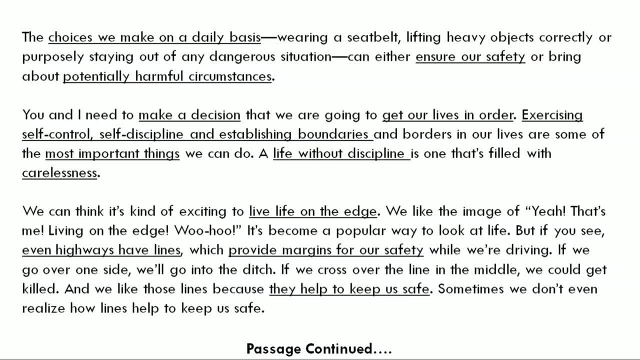 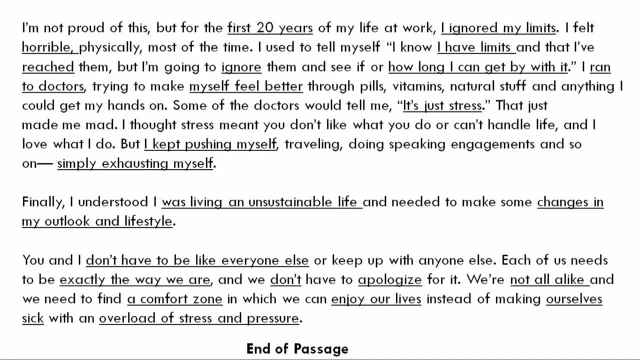 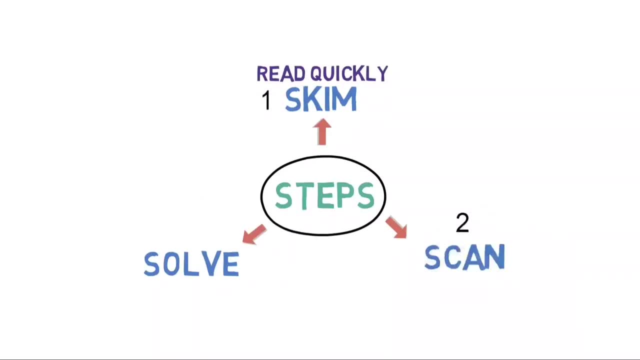 1. the key points in the slides. i will solve some of the questions and give some questions to you to solve. so this is the entire passage. i hope you would have completed the two steps: step one, which is skimming, and step two, which is scanning the passage in detail. 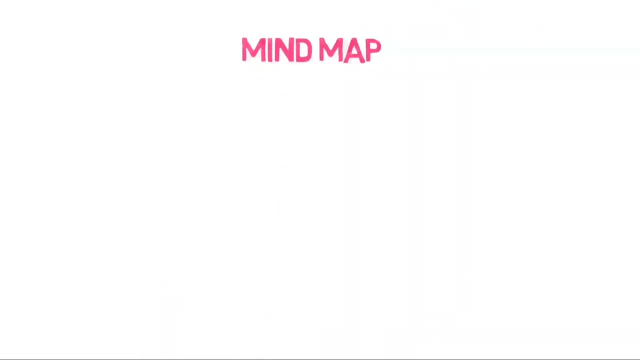 now i will be creating a short mind map. based on my understanding, it is a part of step two. the author explained two ways of living life: balanced life and imbalanced life. he explained what are the ways to live a balanced life and how imbalance can create chaos in life. for balance in life, you must 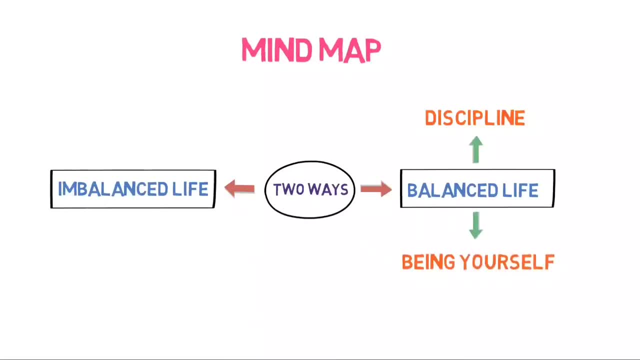 have discipline and have an attitude of being yourself. the author has given an example of lines of highways to explain discipline. the author explained how imbalance created an overburden in his life. constant need of doing something new made him stressful, constantly comparing and trying to become someone else. finally, he concluded that you must have balance in life and to live. 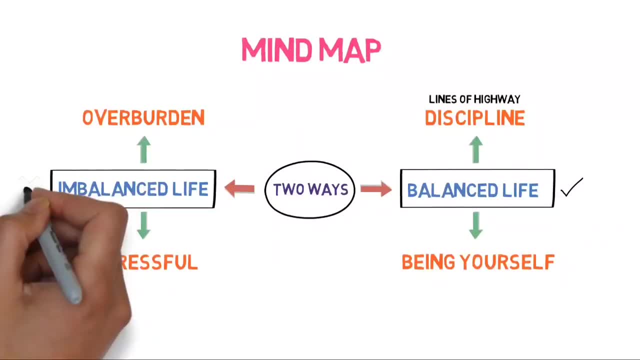 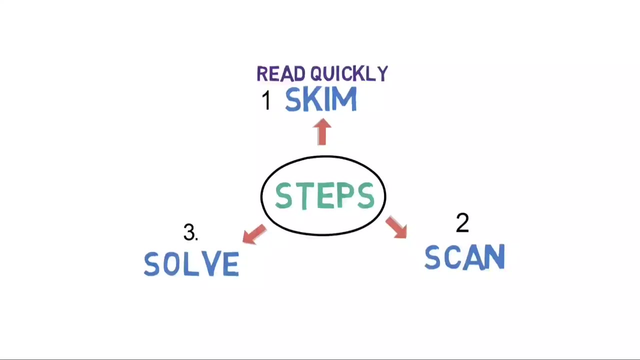 comfortably, instead of living an imbalanced life by an overburden of work. this is the mind map that i created. you may create one if time permits. now let's look into step 3 of our strategy: solve. there are two kinds of questions. number one: here you will have to go to specific text. 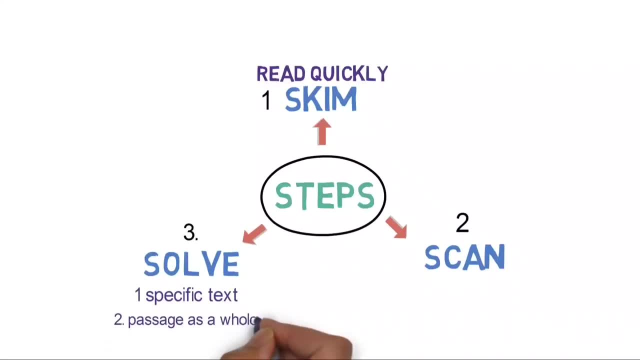 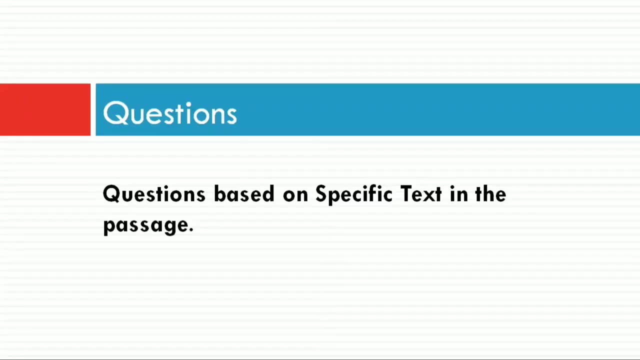 to get the answers- and number two here- you will have to understand the passage as a whole. based on your understanding, you can solve this kind of question first. i have picked the questions based on the specific text in the passage and, for your benefit, i am adding the specific text as well. 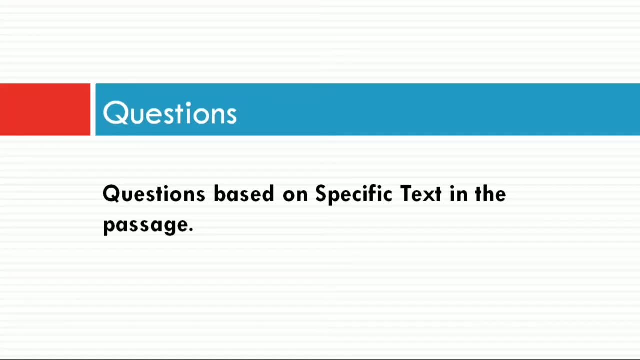 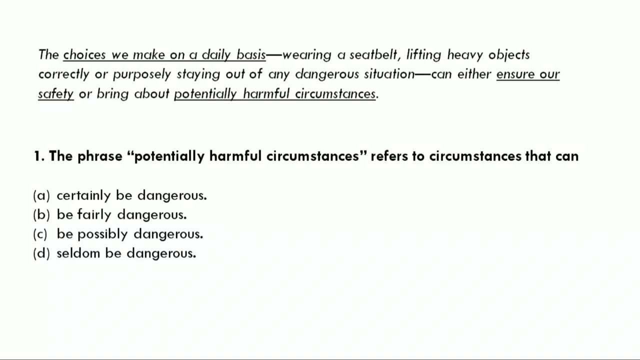 at the top of the slide, so let's start with the questions. number one: the phrase potentially harmful circumstances refers to circumstances that can: a- certainly be dangerous, b be fairly dangerous, c be possibly dangerous and d- seldom be dangerous. if you read the above text again, you will understand that potentially here means possibly. so the correct answer is: 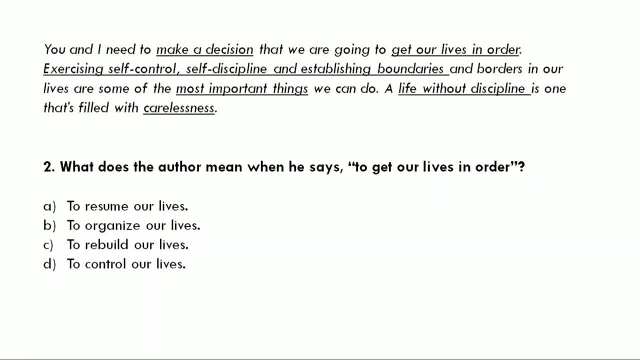 be possibly dangerous. next question, question number two: does the author mean, when he says to get our lives in order, a to resume our lives, b- to organize our lives, c- to rebuild our lives or d- to control our lives? if you read the about text again, you will understand that the author wants us to. 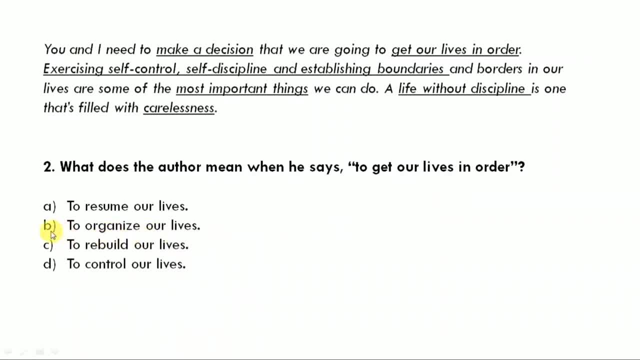 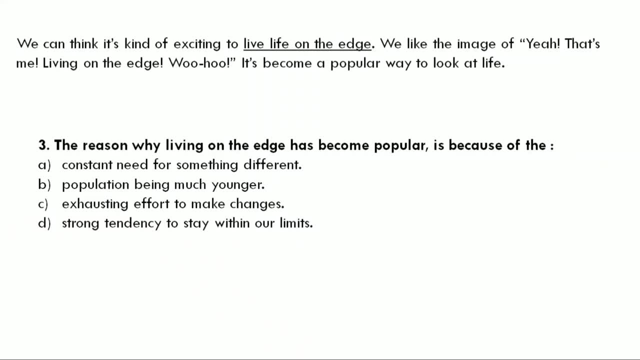 follow discipline. so the correct answer is: b- to organize our lives. next question, question three: the reason why living on the edge has become popular is because of the: a- constant need for something different. b- population being much younger. c- exhausting effort to make changes or. d- strong tendency to stay within our limits. if you read the above text, you will understand. 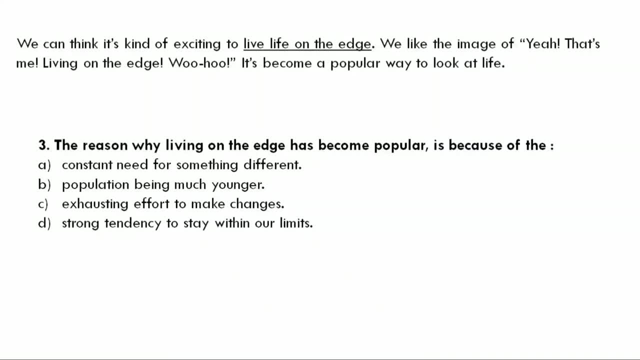 that the reason why living on the edge has become popular is because we need something new all the time. here the answer is not given directly, but the meaning is implied, so the correct answer is option a constant need for something different. next question, question four, the author uses: 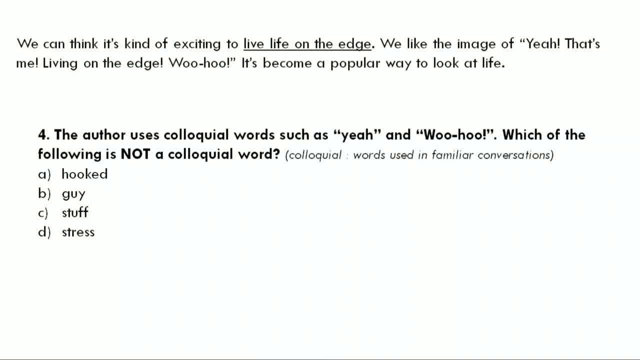 colloquial words such as yay and woohoo. which of the following is not a colloquial word? here you must know the meaning of colloquial to solve this answer. colloquial means used in ordinary or familiar conversation, not formal way. so here the correct answer is stress. 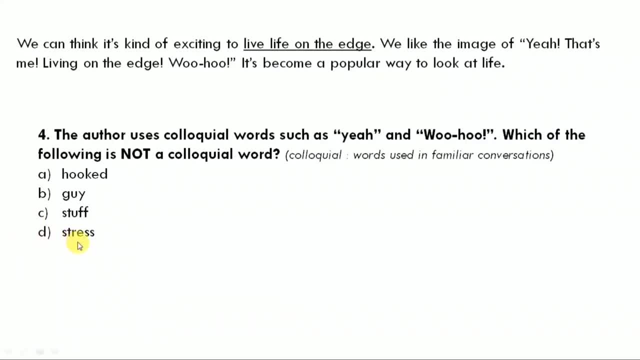 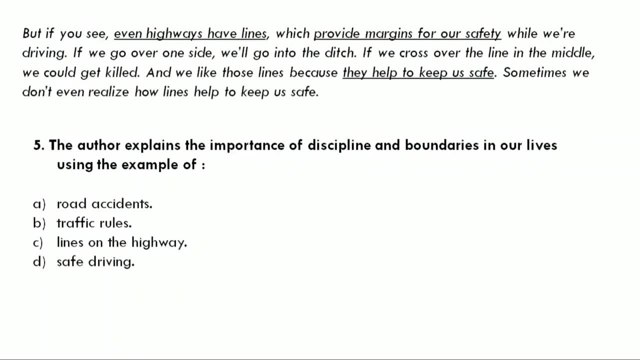 as we use it formally, rest. all other words are colloquial words, including hooked guy and stuff. next question, question five, the author explains the importance of discipline and boundaries in our lives using the example of a road accident, b- traffic rules, c- lines on the highway or d- safe driving. if you read the above text again, you will understand. 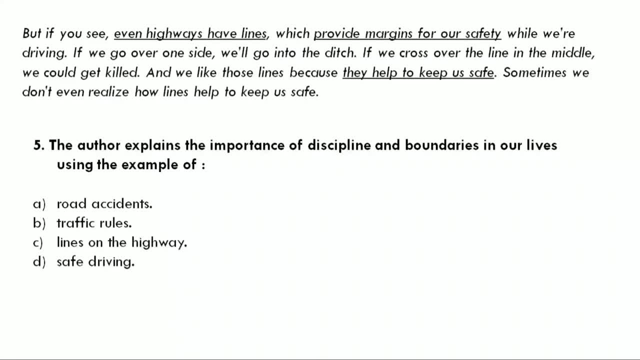 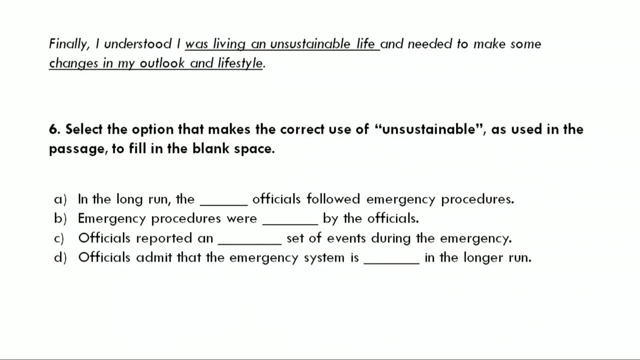 that the author explains the importance of discipline with the help of c lines on the highway. so the correct answer is c- c lines on the highway. next question, question six: select the option that makes the correct use of unsustainable, as used in the passage to fill the blank space. 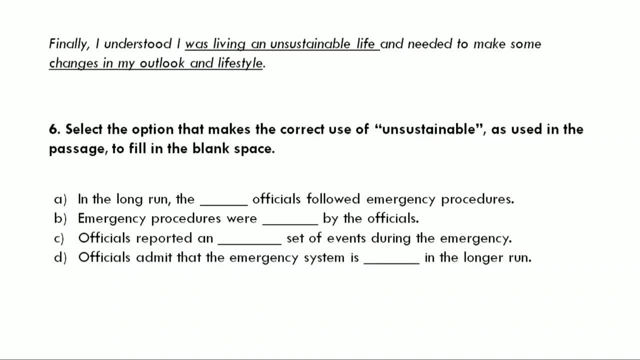 unsustainable means unsustainable, as in the passage to fill the blank space. unsustainable means something that cannot be continued for a very long time. if you read carefully, you will find that the correct answer is option c. officials reported an unsustainable set of events during the emergency, so these questions were such that you had to read a particular text again from the. 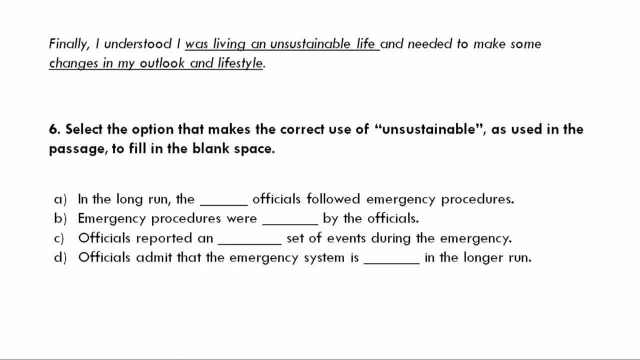 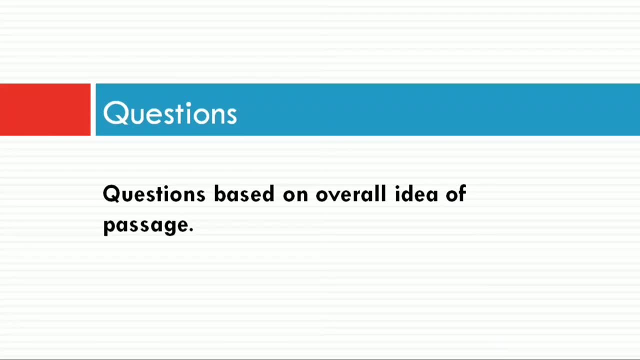 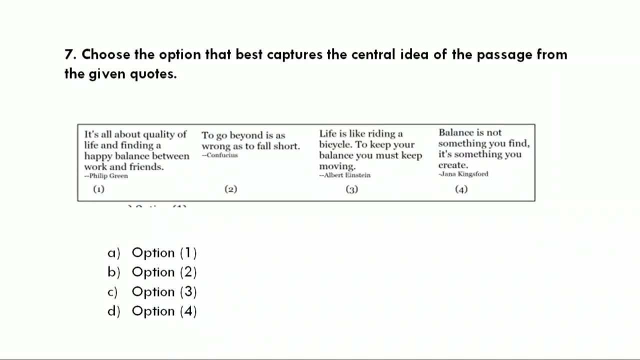 page to solve the answers now. the next set of questions are such that you can solve them only if you understand the overall idea of the passage. so let's look into it. question 7: choose the option that best captures the central idea of the passage from the given quotes. the main essence of the 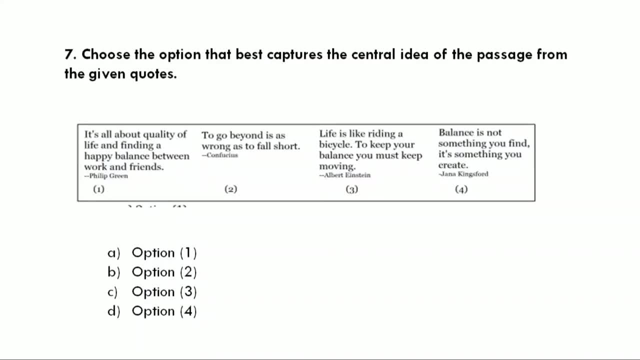 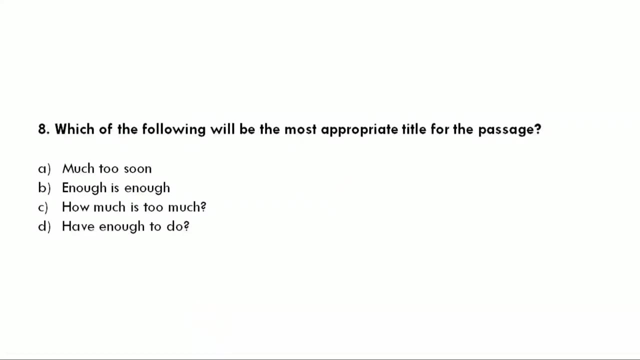 passage is to understand and create a balance in life, so the correct answer will be option d: balance is not something you find, it is something you create. next and the last question is question of the following: will be the most appropriate title for the passage? a- much too soon. b- enough is. 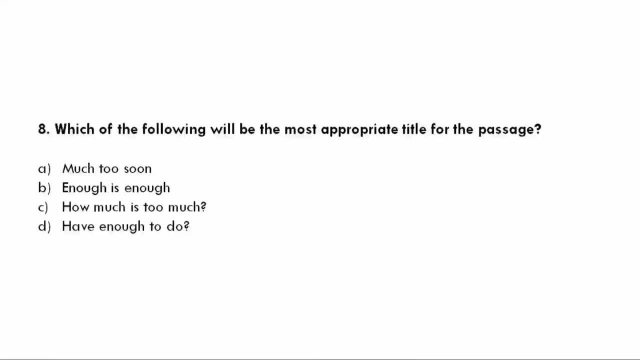 enough. c- how much is too much? or d- have enough to do. option c is the correct answer as it brings out the true meaning of the passage, as it is about deciding the extreme limits of our comfort zone to lead a balanced life. i hope now you are clear on how to solve this type of question. 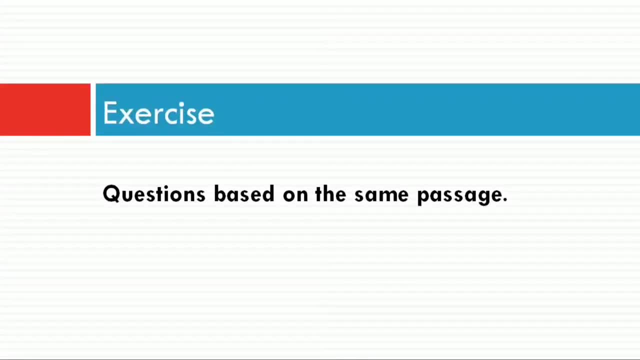 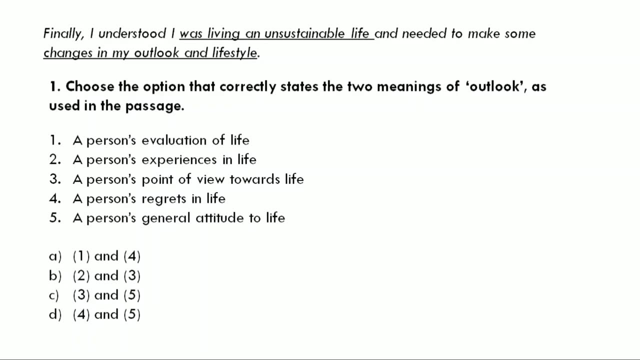 now i am giving you an exercise to practice from this passage only. the first question is: choose the option that correctly states the two meanings of outlook as used in the passage notice. i have added specific text at the top to help you figure out the answer. let's look into the next question. 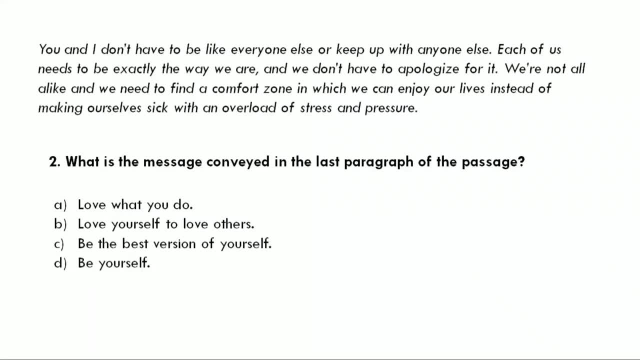 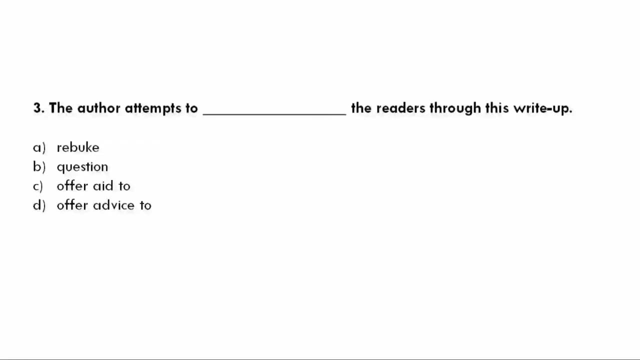 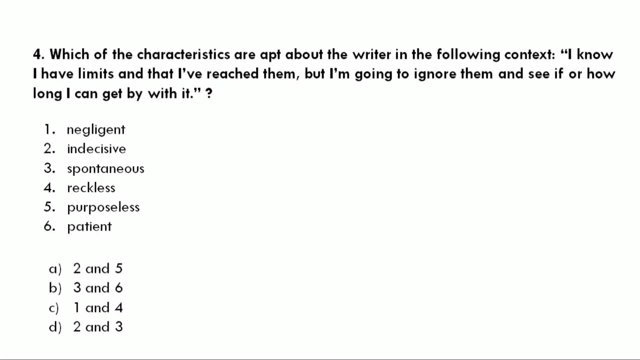 question 2: what is the message conveyed in the last paragraph of the passage? love what you do, love yourself to love others. be the best version of yourself or be yourself. question 3: the author attempts to dash the readers through this write-up rebuke question, offer aid to. and the last question: which of the characteristics are? 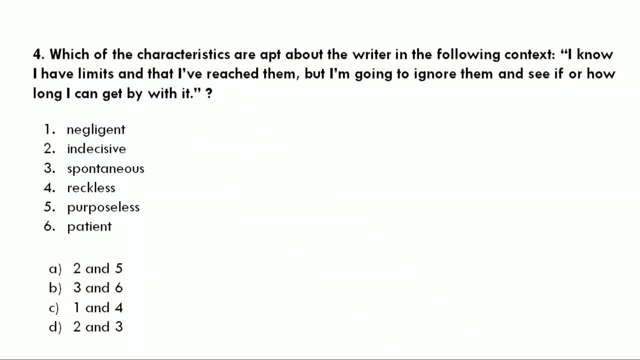 apt about the writer in the following context: i know i have limits and that i have reached them, but i am going to ignore them and see if. for how long can i get by with it? please write your comment section. i will be waiting for your reply. let's quickly revise what we learned in this. 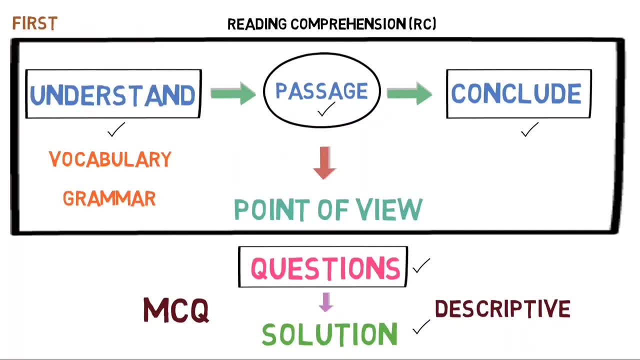 lesson. first, we understood what is reading comprehension. reading comprehension is the ability to understand the content of the given passage and to draw a conclusion from it. here the author will give his point of view from different angles for a particular topic and you have to draw out a conclusion from it to test what you have comprehended or understood. for